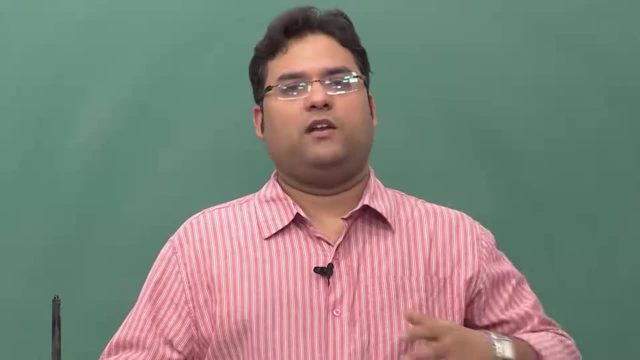 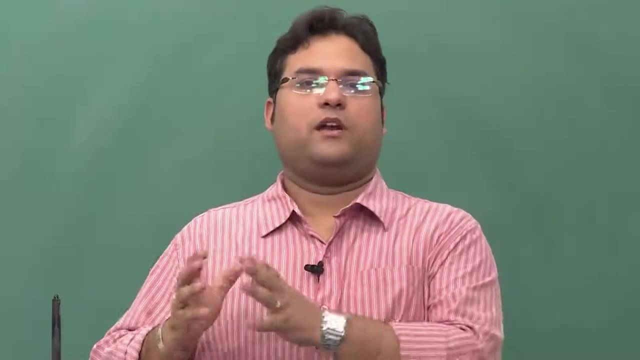 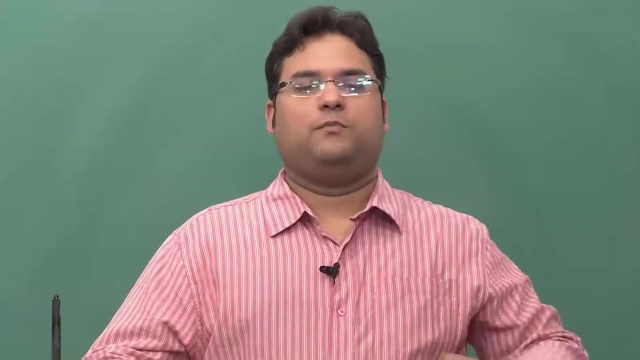 So that is why I am saying that I am following the convention here, But we will begin with understanding more details about Visual Perception in the end and, if time permits, we might talk about Auditory Perception and related processes as well. That said, we will talk about the basic part, or 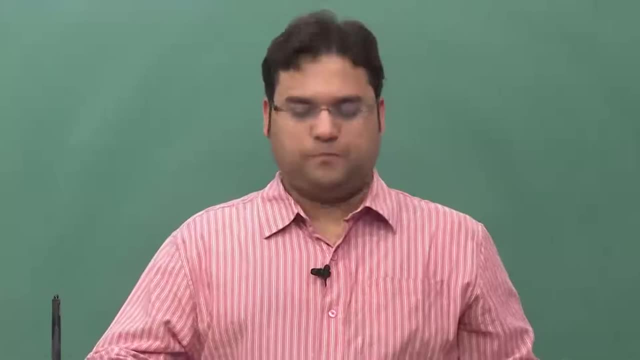 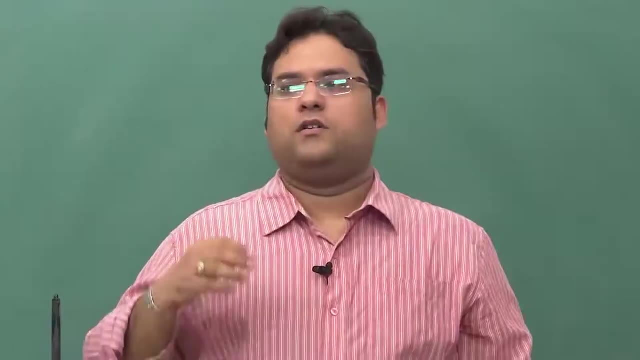 the first entrance into what Visual Perception as a process is like. So how does this really begin? We will try and understand the Physiology of Visual Perception, The function or say, for example, how do our eyes see? What really helps our eyes see? 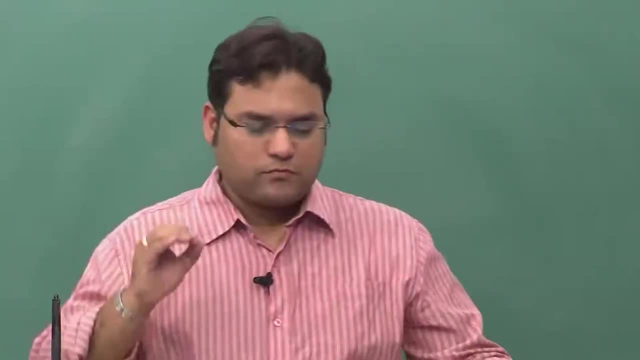 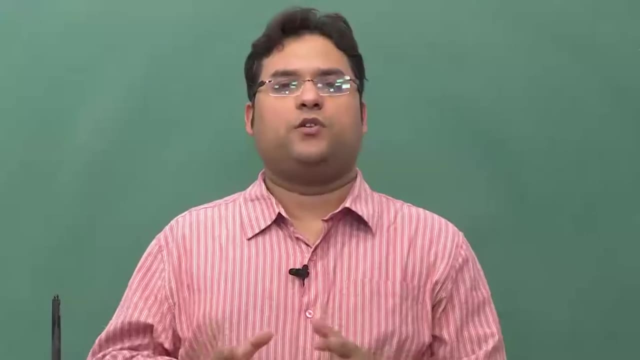 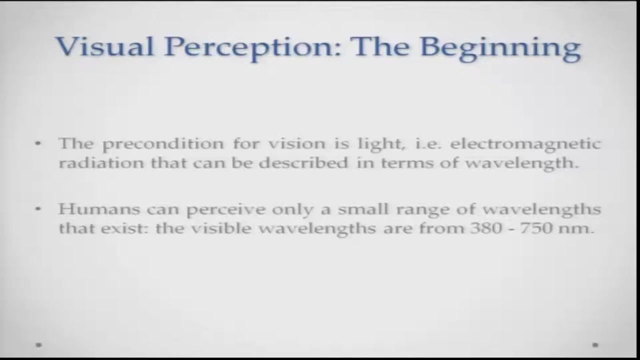 And what are the very basic processes. I am not going to go into a lot of detail about each of these. The idea is just to give you a flavor of what are the constituent processes in Visual Perception. So let us begin. The beginning point, or the initiating point of Visual Perception is: 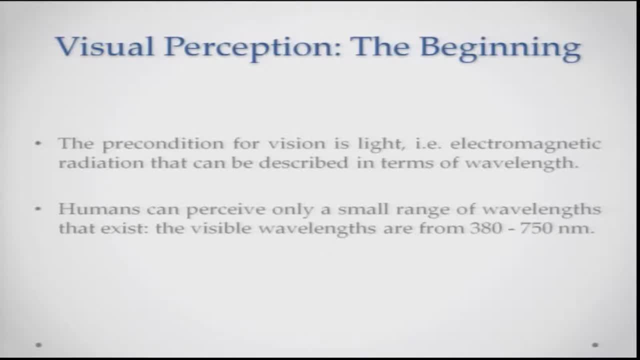 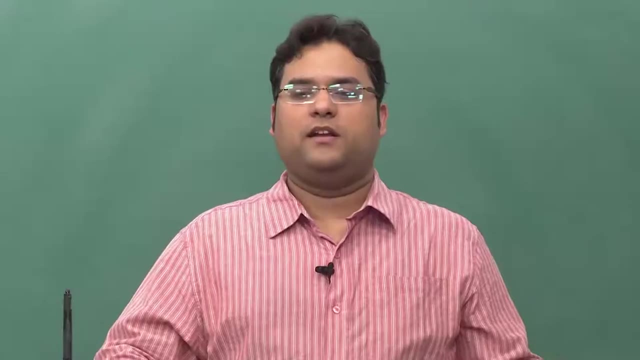 basically the registering of light in your eyes. So the precondition for the fact that you can see- anything for that matter- is the presence of light. If there is light, you see. If there is no light, you do not. So it is kind of a sort of a binary there. Now, what is light? Light is basically 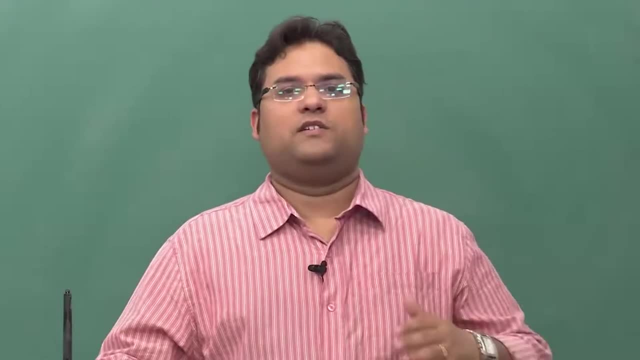 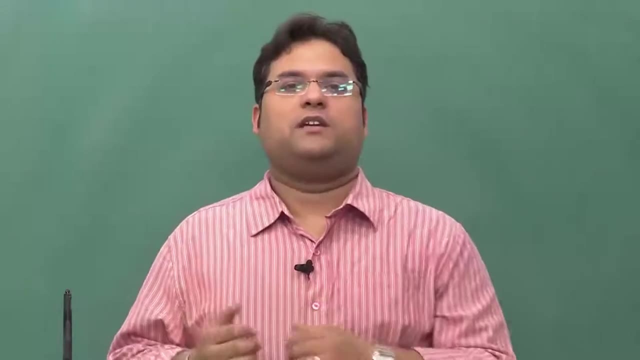 electromagnetic radiation that can be physically described in terms of wavelength. There is this range of wavelength which we are most familiar with, So the range of wavelength which we are most sensitive to, and that basically forms what is called Visible Light for us Humans can perceive. 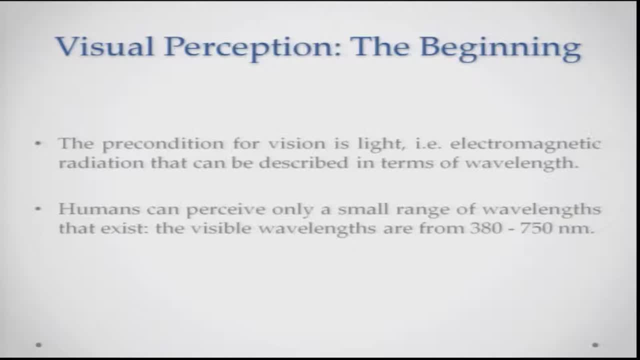 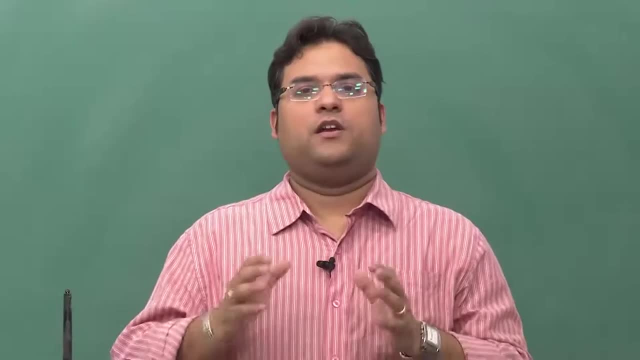 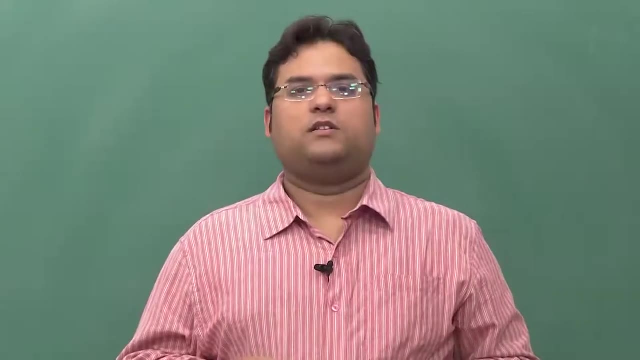 only a very limited range of this wavelength, of this Electromagnetic Radiations, and this Visible Wavelength basically falls between 380 to 750 nanometers. Here you can see the range of visible light. So there is this Electromagnetic Radiation here. It isippled light with a. please watch the video and learn. 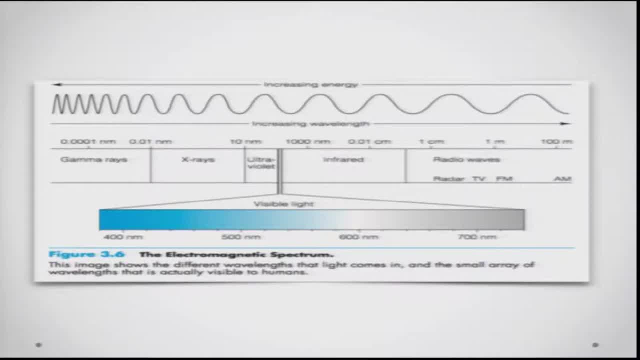 watch the program, Then we welcome our next step ofLEARN DELEARNEDGER. So next step, we are going to electromagnetic radiation, and right from 380 nanometers to 750 nanometers is what we can actually see. So any electromagnetic radiation or the electromagnetic radiation in this wavelength is what constitutes. 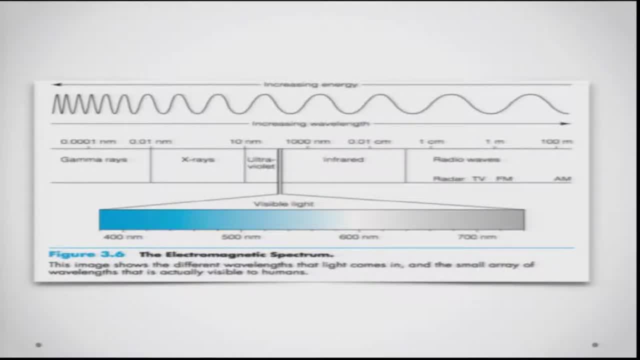 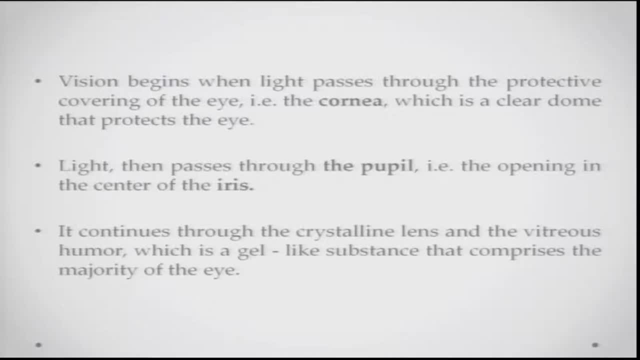 our, you know, visible spectrum. Now, how does the process of vision really begin? where does this, you know, how does light contribute to us seeing? So, vision, basically, or our, you know, sensation of anything in this world through the eyes? 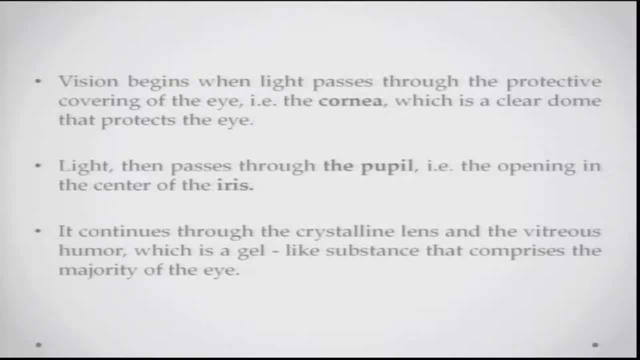 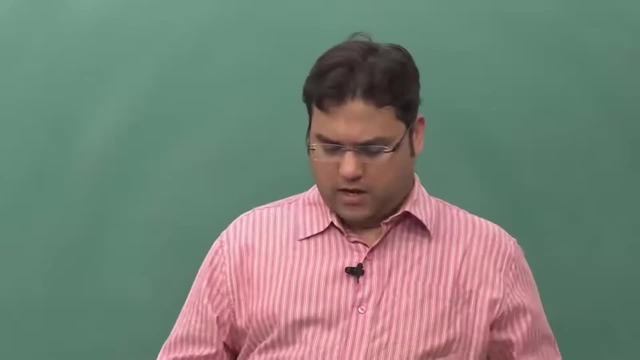 start when light passes through this protective covering of the eye, the top part of the eye, which is the cornea, which is a clear dome that protects the eye. We will talk about that. I can actually show you the figure and come back here. 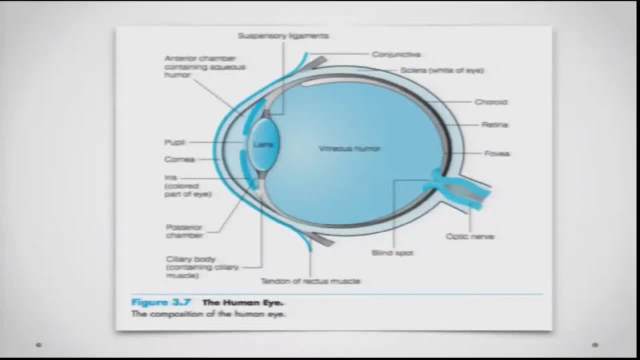 This is what the eye actually looks like. You can see there are these different parts here. You can see that there is a pupil, there is cornea, there is a part called iris, there is a posterior chamber wherein the lens is situated, and then there is this ciliary body. 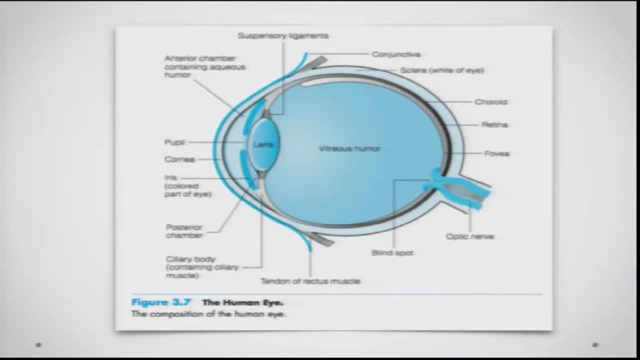 which has those muscles. The eye is filled with some substance which is called the vitreous humor. At the back you can see there is things like the retina, there is the fovea and there is an exit nerve which is called the optic nerve. 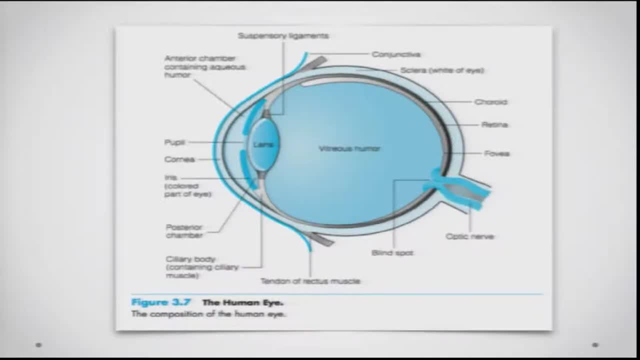 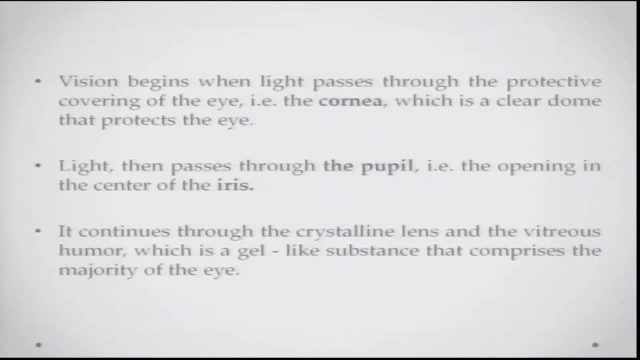 So, again, I am just taking names of these different areas. we will talk about them in much more detail as we go ahead. Now, what is so? you can see what is the cornea. Cornea is basically a clear dome that is protecting the eye, something that is the 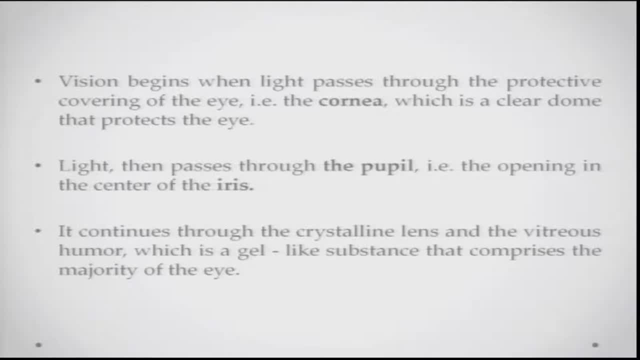 outer layer of the eye. Then through this cornea the light passes through the pupil. Pupil is basically the opening in the centre of the iris. You can again refer to the figure Here. you can see that there is this pupil, which is the opening, you know, in that thing. 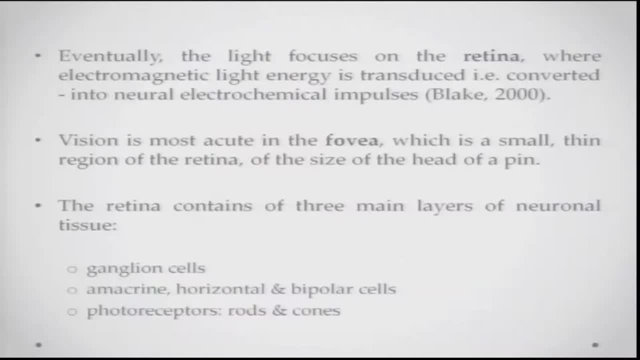 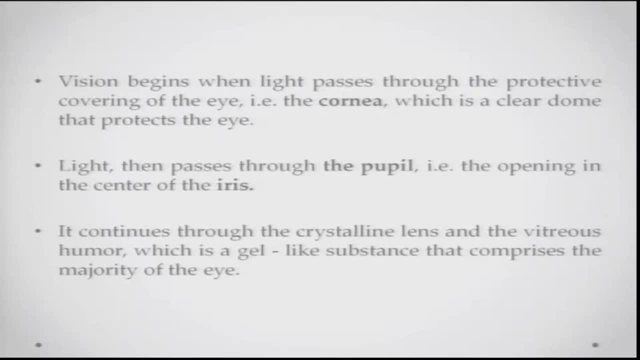 called the iris. You can see that already in the figure, So light kind of. so it starts through the cornea, Passes through the pupil, which is basically the opening in the centre of the iris, and then it continues through this crystalline lens which you saw and the vitreous humor. 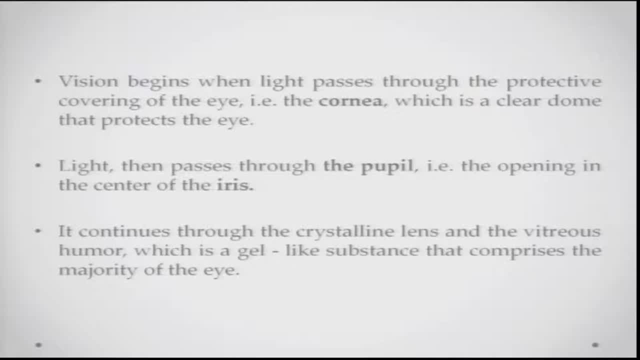 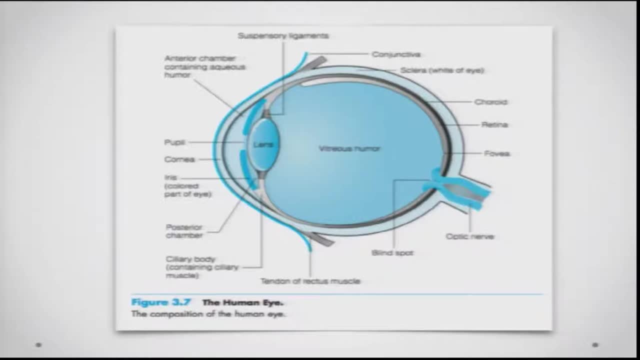 which is a gel like substance, which is filled in the eye and then it reaches at the back. So you see, the eye starts at the cornea, goes through the pupil, passes through the lens, passes this entire gel, like vitreous humor, and goes at the back. 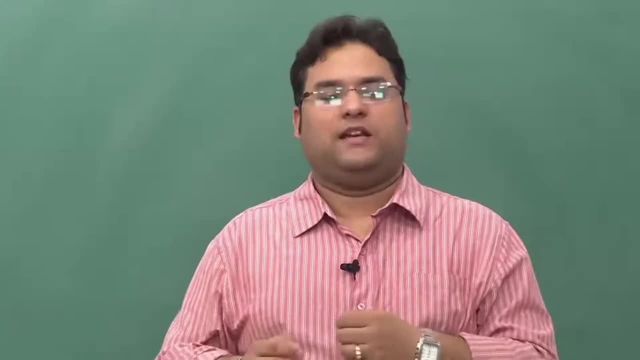 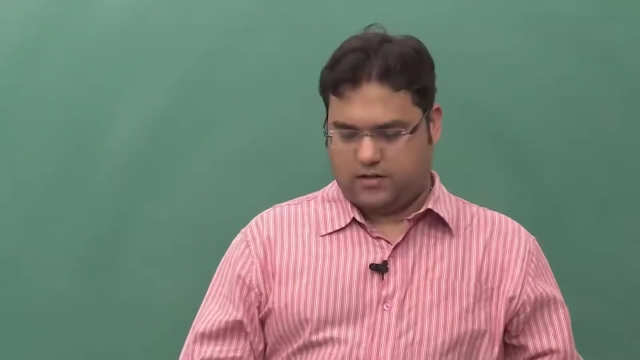 At the back is where the real processing of the light starts. So let us go ahead, Let us go ahead, Let us go ahead. So the light then focuses on what is called the retina. You might again refer to the figure. 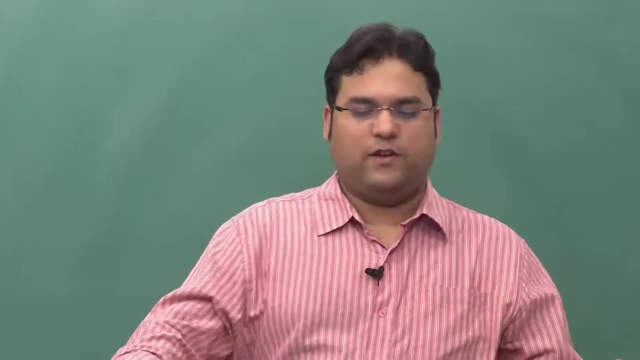 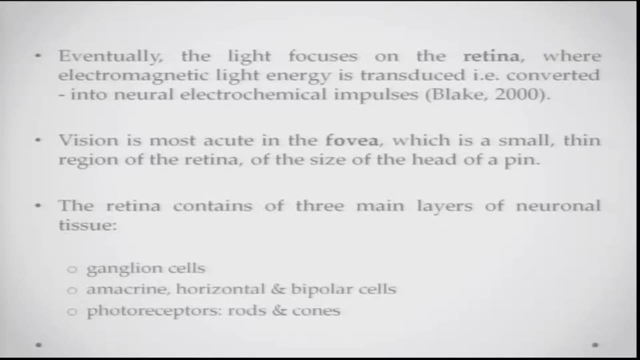 At the back there is this retina. Retina is basically where the electromagnetic energy, that is light, is transduced, that is converted into neural electrochemical impulses. If you are interested in what transduction is, any signal from the external world, you might remember in the psychophysics class we have talked about it. 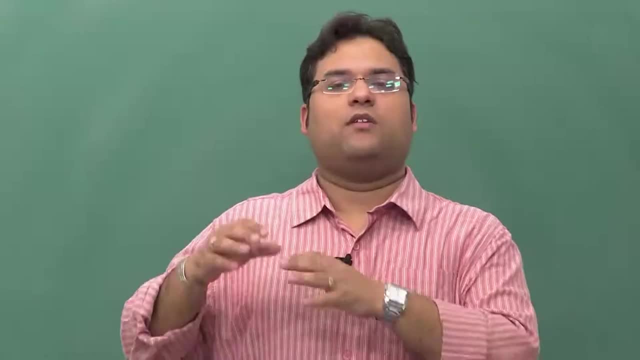 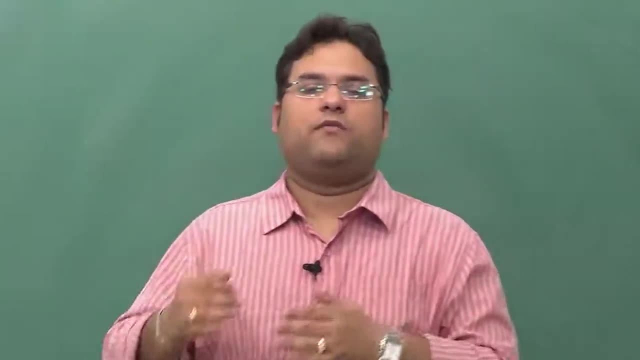 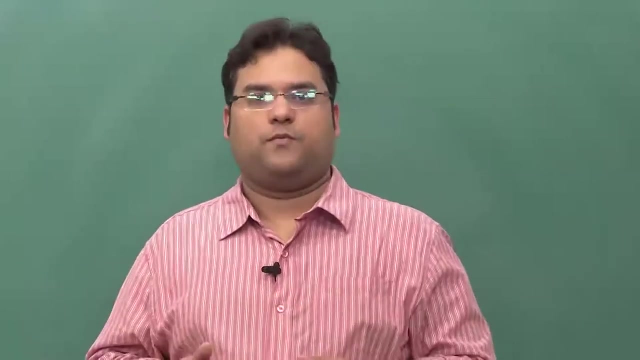 Any signal from the external world, any sensation, needs to be converted. It needs to be converted into a signal that can be understood by the brain. So the electromagnetic radiation, which is light, needs to be converted into neural impulses so that the eyes, or the brain, more importantly, can make sense of it. 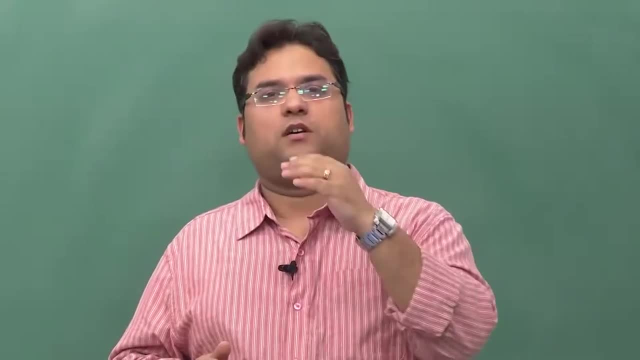 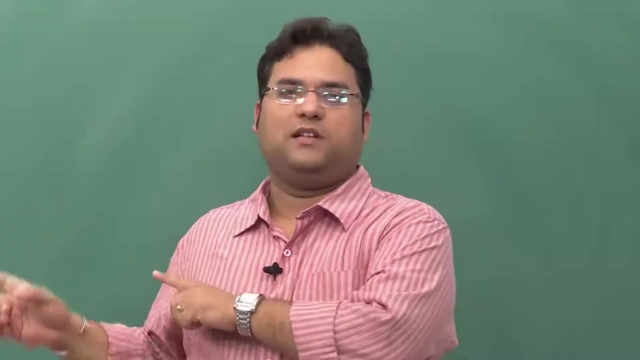 So the light passes through the cornea, goes through the pupil, passes the lens and the vitreous humor goes and falls back at the retina. At the retina is where this is converted into electrical impulses. That is where the brain starts making sense of this. 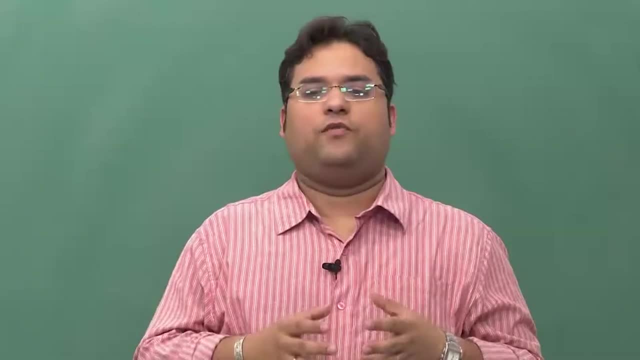 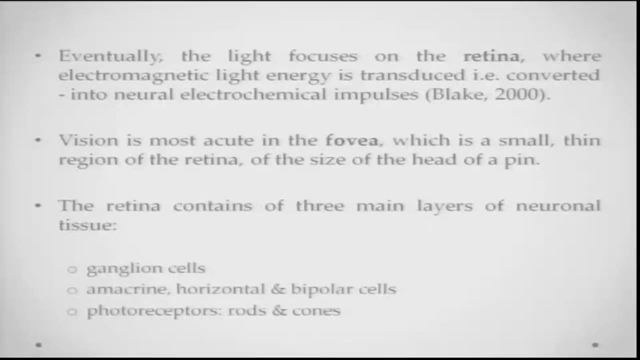 The vision is most acute at the fovea. The fovea is a very small, thin region of the retina which is basically at the size of a pen, just like the size of the head of the pen. The retina basically contains layers of neuronal tissue. 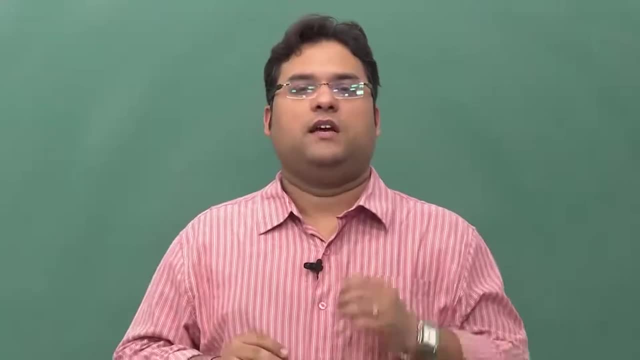 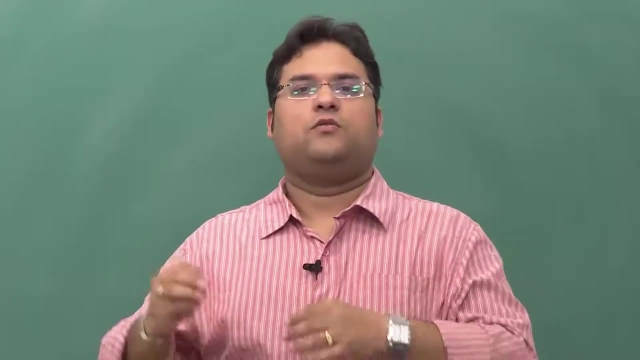 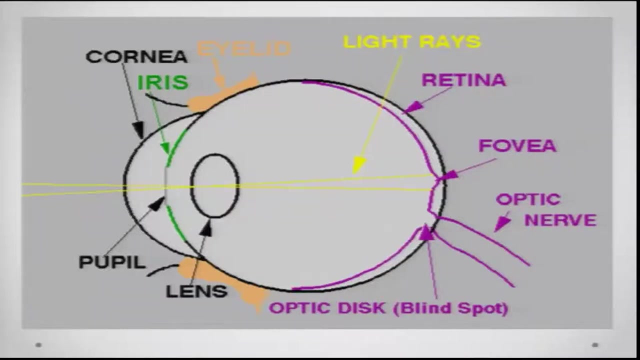 These neuronal tissue basically includes different kinds of cells, cells like the ganglion cells, the amacrine cells, horizontal cells, bipolar cells and then also photoreceptor cells called the rods And the cones. We will ah. So here you can see a more clear picture of the cornea, the iris. you see the pupil. 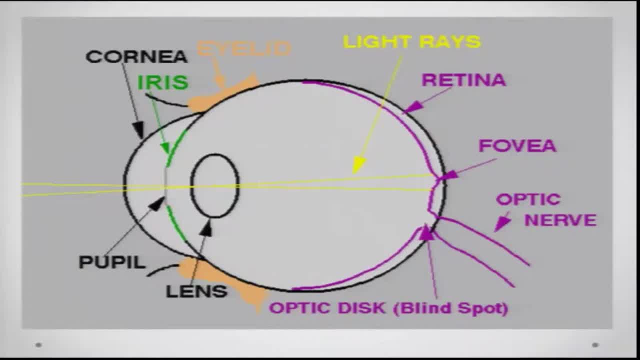 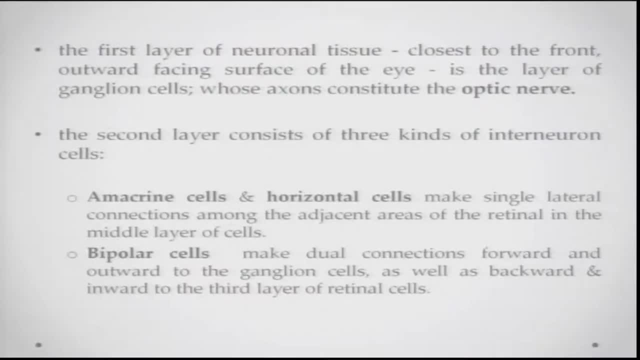 is there. there is the retina at the back and you will see that bulge, ah, just like a pin, the head of the pen, that is what the fovea is Here. ah, there is this layering of these different kind of cells. So the first layer of the neuronal tissue at the retina is closest to the front outwards. 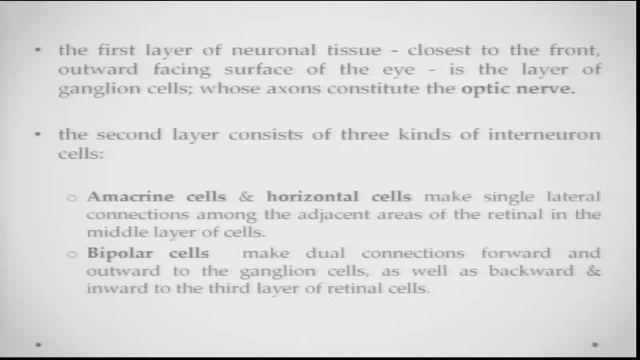 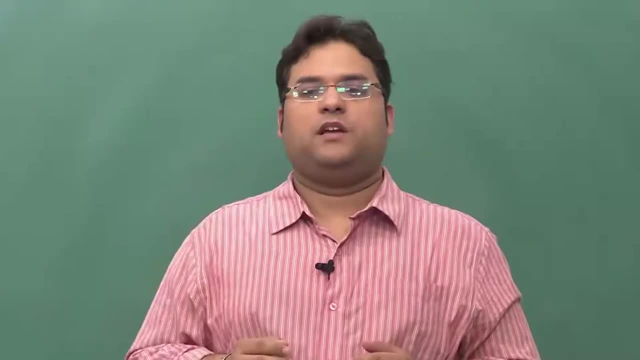 facing surface of the eye. So the first layer is the ah layer, ah, which, ah, You know, the light falls first. so outwards, ah, facing surface of the eye. This first layer is basically, ah, the layer of what is called the ganglion cells. ok, 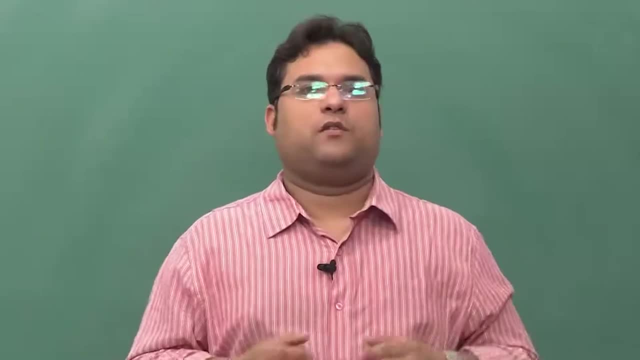 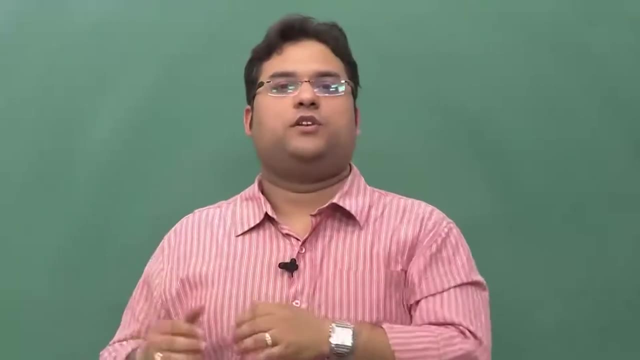 The axons of these ganglion cells. if you remember the ah chapter on perception, the axons are actually the ah part which kind of protrudes from the cell body. The axons of these cells constitute ah, combined together to form what is called the optic. 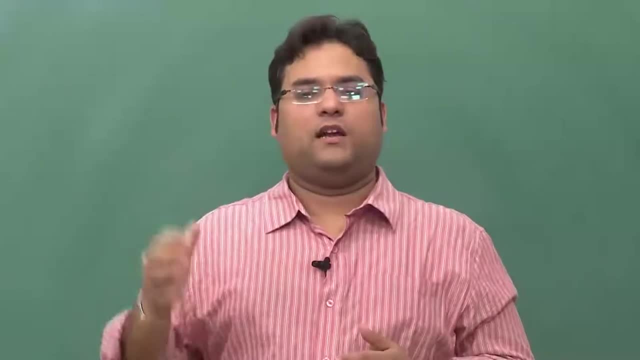 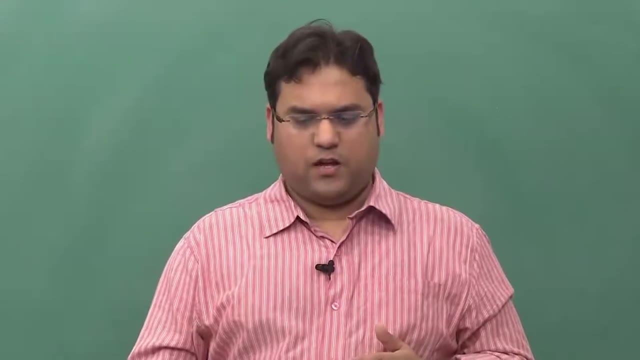 nerve. So this, this is the outer ah facing surface of the cell, the ganglion cells which form the optic nerve. ah, I will show the show, the figure, to you. ah, now, ah, So you can see that. see, there are these ganglion cells ah, in the ah layer number 3, the axons. 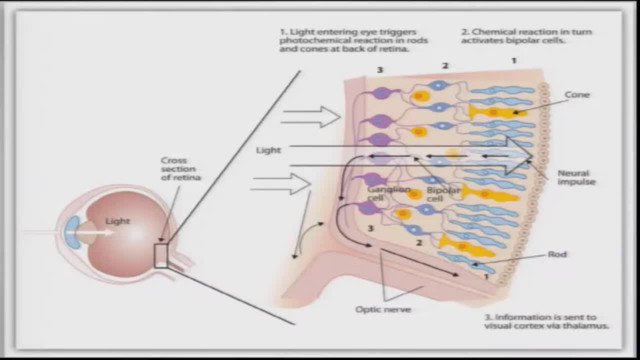 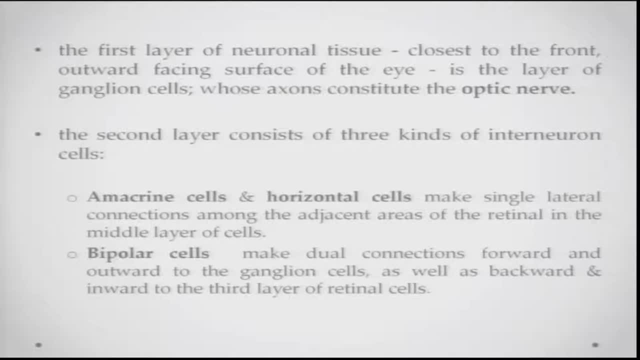 of which are forming what is called the optic nerve. ok, ah, Coming back, the second layer consists of three kinds of interneuron cells, ah. These cells are the amacrine and the horizontal cells and the bipolar cells. The amacrine cells basically make single lateral connections. 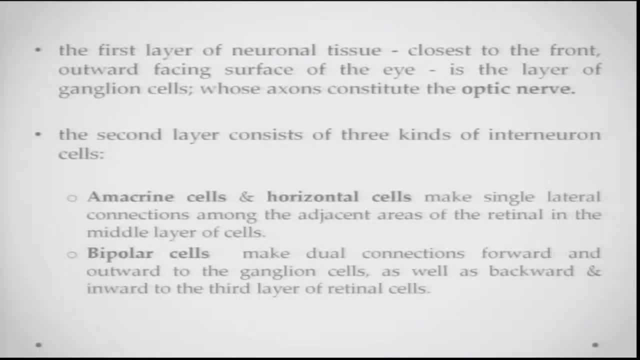 So this is the amacrine. The amacrine cells are the connections to adjacent areas of the retina ah. in the middle layer of the cells, The bipolar cells make dual connections. They make connections forward and outward to the ganglion cells, as well as backward. 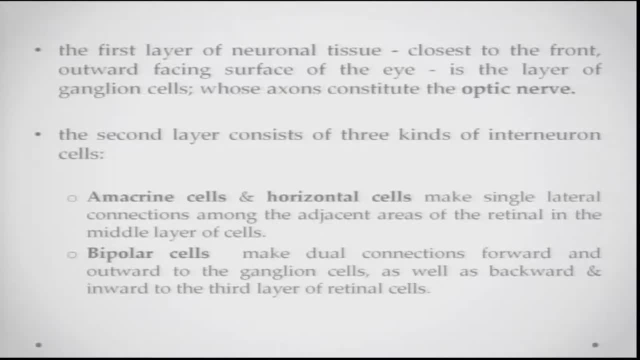 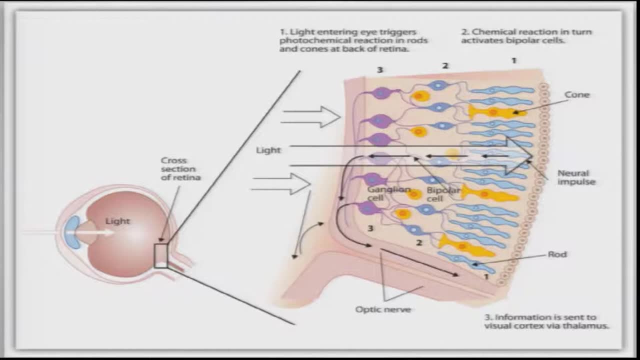 and inward to the third layer of these retinal cells. So you will see these connections now. ah, you can see the bipolar cells being connected to the inward- ah, ah, rods and cones- and also to the ganglion cells. So they are basically connected to both inside and the outside part. 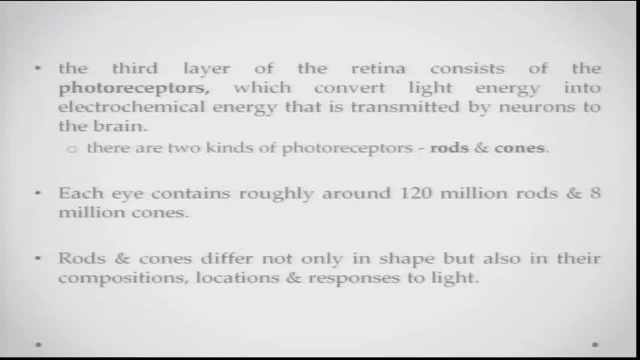 Ok, is basically the layer which consists of what are called photoreceptors. As you can guess from the name, these are the cells which basically convert light energy into electrical energy that is transmitted by the neurons to the brains. So this is where exactly this process of transduction is. 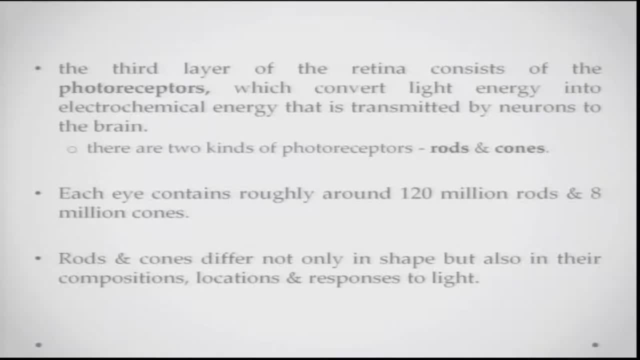 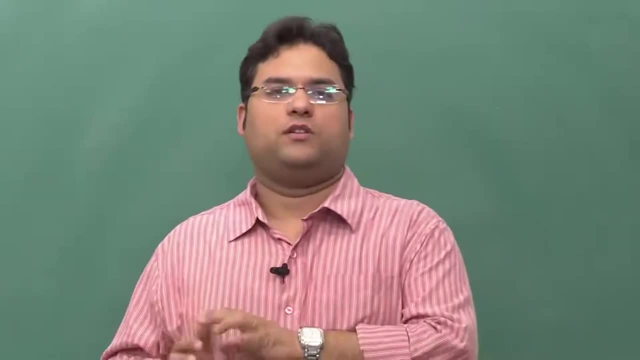 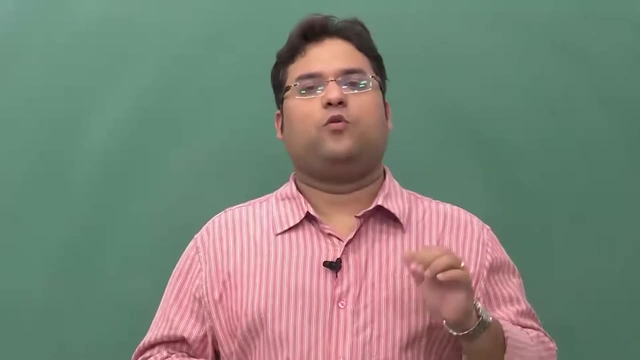 happening. There are two kinds of photoreceptor cells: rods and cones. Each eye consists about 120 million rods and around 8 million cones. Both of these cells have their own specialties. I will talk about them in just a moment. Now, rods and cones simply do not only differ in shape. 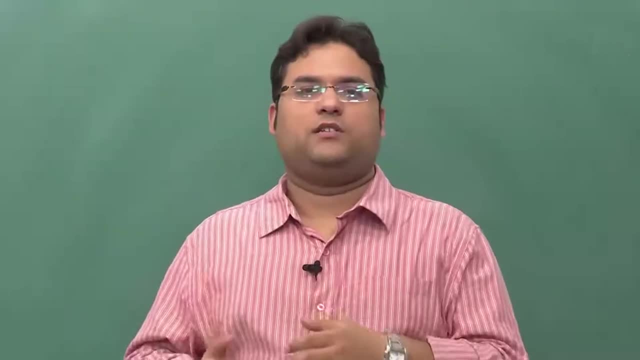 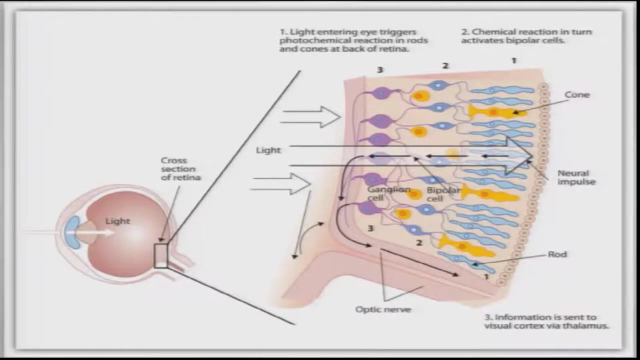 but they also differ in their compositions, what they are made of, their locations and how they respond to light. Before we go further, it might be helpful to see these cells again. So you see that there are three layers: The first layer, or actually the third. the layer number three is: 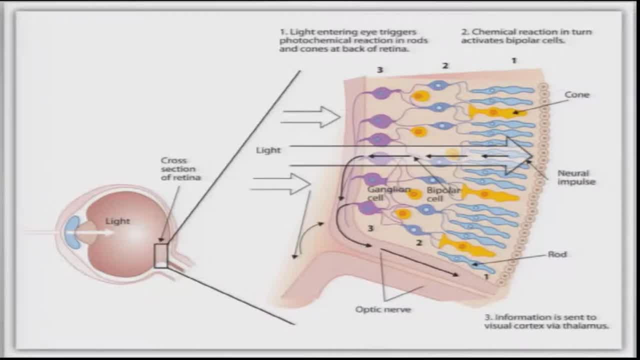 basically your ganglion cells. The layer number two is the ganglion cells. The layer number two is your bipolar cells, connected both inwards and outwards, And the layer number one is basically your photoreceptors. You can see the rods and cones in different shapes there, So you can see. 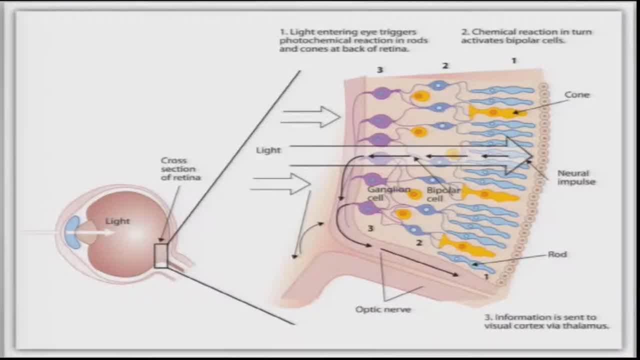 how light is really moving. Light is energy, is entering the eye and it is triggering photochemical reactions in rods and cones at the back of the retina. Chemical reaction in turn activates the bipolar cells. From the bipolar cells, information is going to the ganglion and from there it is. 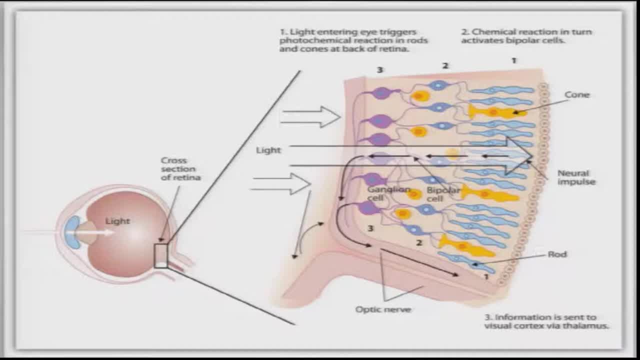 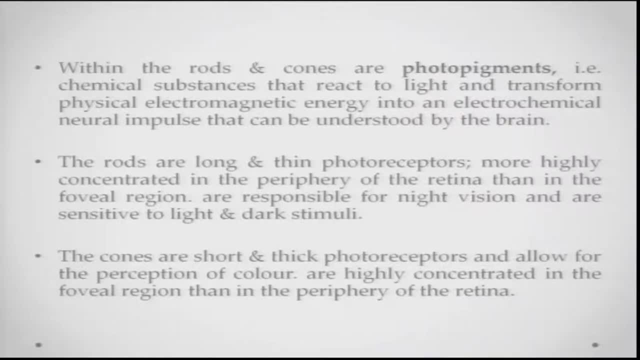 going to your optic nerve and via the optic nerve it is going to the ganglion. So this is the optic nerve It actually transmits to the brain. Now, what are these rods and cones doing? These rods and cones basically have substances which are called photopigments. Photopigments are chemical. 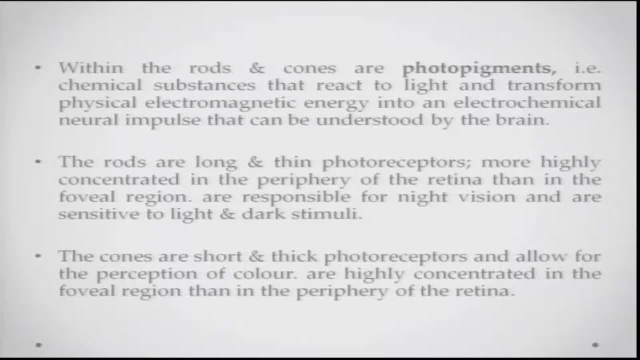 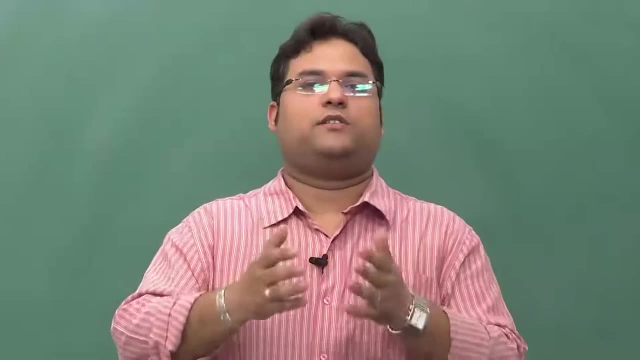 substances that react to light and transform physical electromagnetic energy, which is light, into an electrochemical neural impulse that can be understood by the brain. Now, electrochemical neural impulse: we have talked about this in the physiology part where we were talking about the reaction potentials and those kinds of things. The rods are long and thin. photoreceptors. 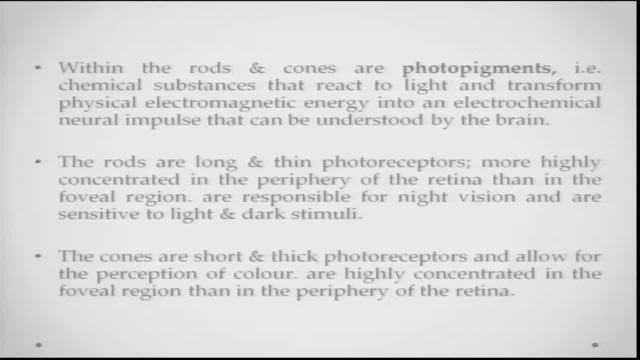 more highly concentrated in the periphery of the retina than in the foveal region. So, rods, you will find they are more concentrated in the outside regions of the retina and they are basically responsible for night vision and are sensitive to light and dark stimuli. 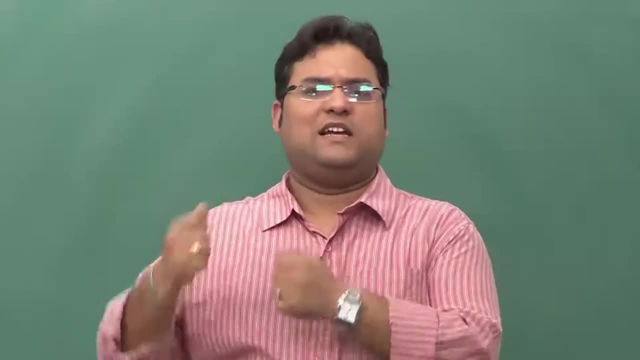 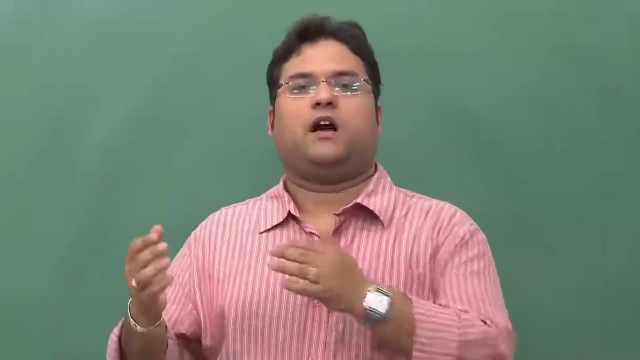 So rods are basically which are more useful when you know there is less light, in night kind of scenarios, because they are basically reacting in binary to whether there is light or whether there is darkness or absence of light. The cones are very short, They are. 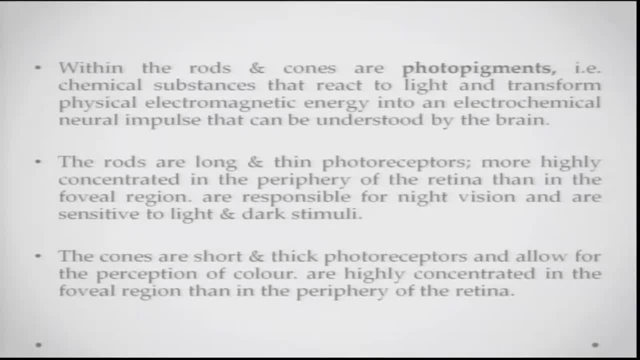 slightly thicker photoreceptors and they allow for the perception of colors. They are highly concentrated in the foveal region than in the periphery, because this is where the light is focused more. This is where the acuity of understanding, of really seeing shapes really. 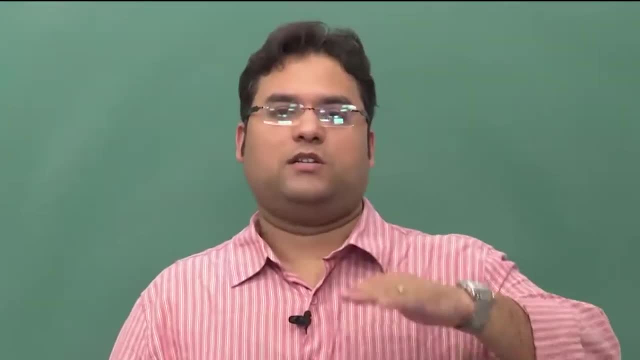 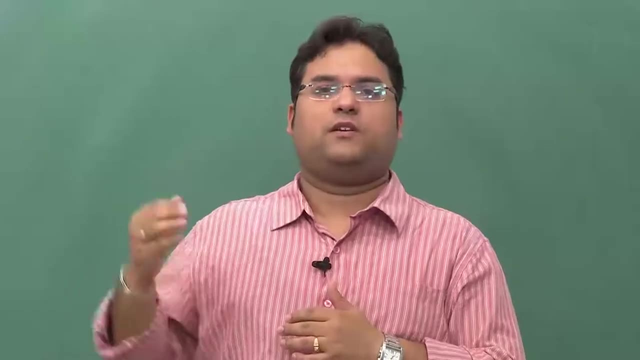 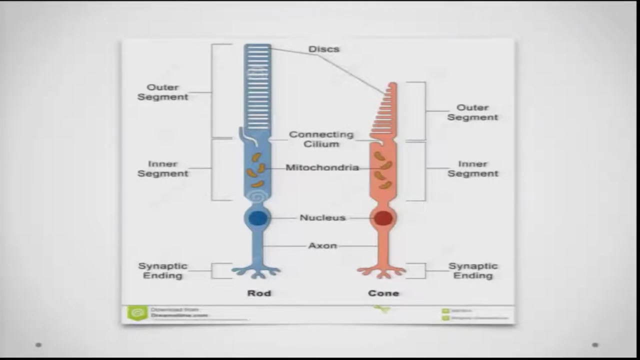 seeing colors is best. So the rods are more sensitive to black and white. The colors are more sensitive to different. Cones are more sensitive to different kinds of colors. Here you can see the difference. basically in rods and cones, You will see. they are not only. 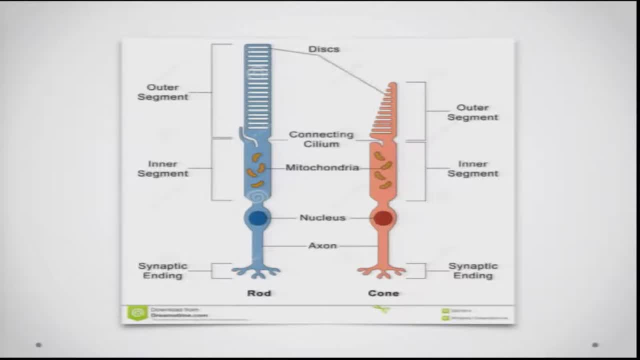 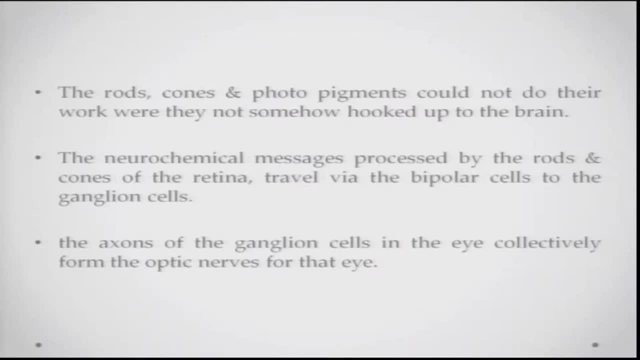 structurally different and they are also functionally different. as we discussed already Now, the rods, cones and the photopigments could actually not do their job if they were not really connected somehow to the brain. So we have to talk about how all of this really connects to. 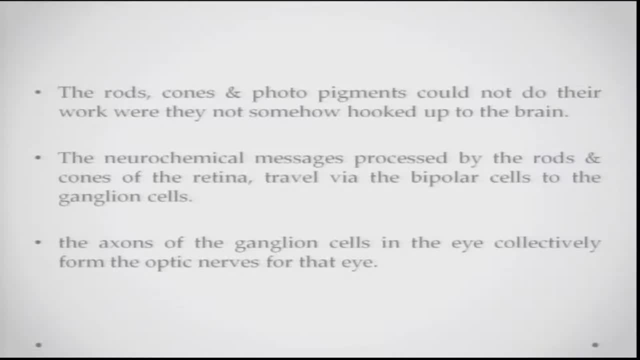 the brain as well. So the neurogenesis of the brain is very important. So the neurogenesis of the brain is very important. So the neurogenesis of the brain is very important. Now you can see that memos that are still produced in the brain, or even nodal Would, 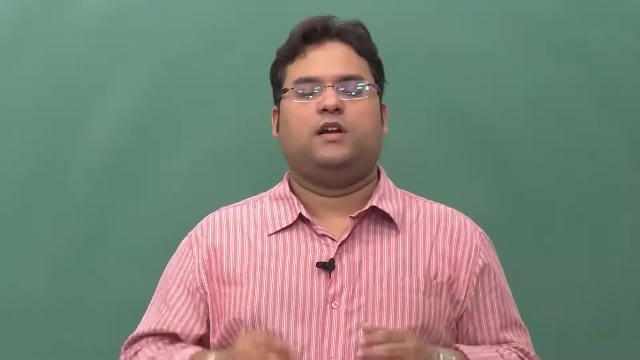 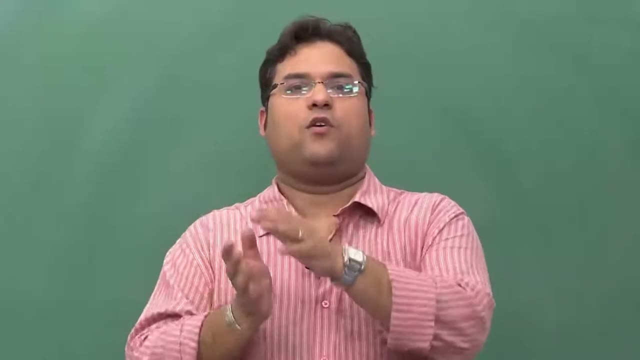 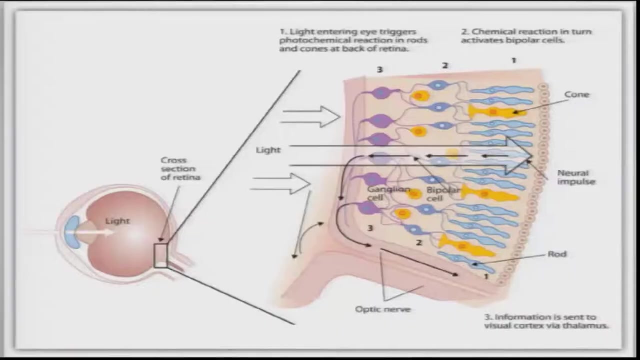 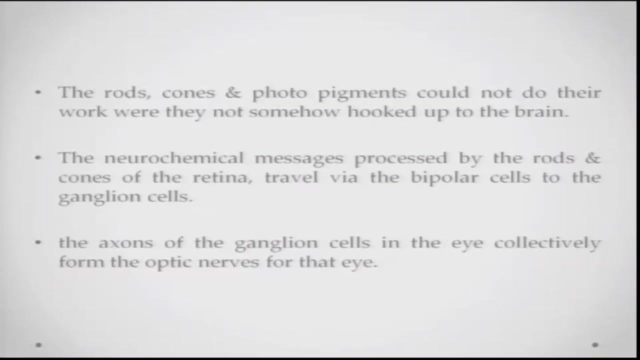 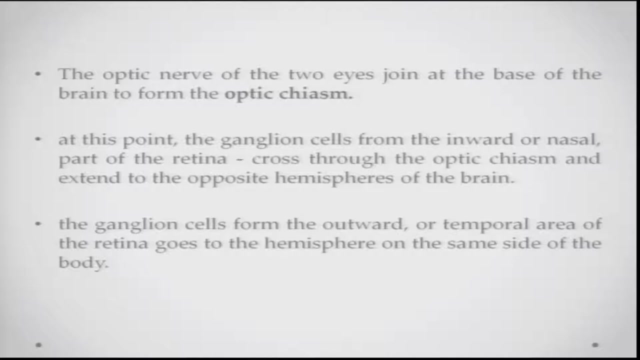 you like to raise your hand? to raise your hand, ło warm, warm, warm, warm, warm, Robinson, on раж join at the base of the brain to form something called the optic chiasm. The optic chiasm, basically, or at this point, what happens is that the ganglion cells from 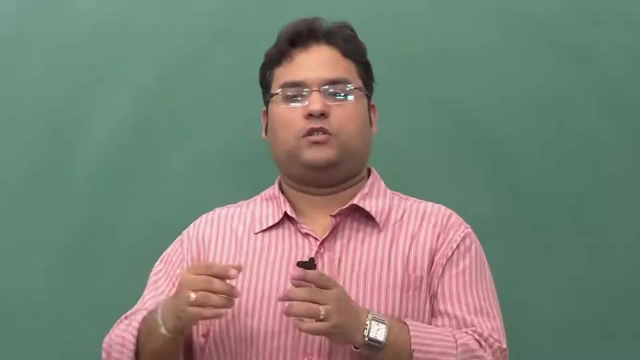 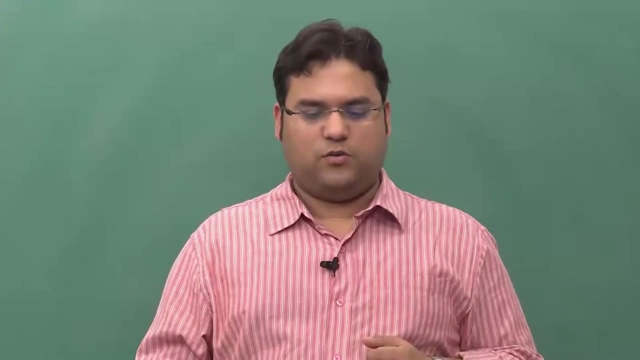 the inward or the nasal part of the retina cross through the optic chiasm and extend to the opposite hemisphere of the brain. So, for example, I can show you, show this to you through this figure. you can see this figure here. you will see that there is an inward or nasal part and there is an outward. 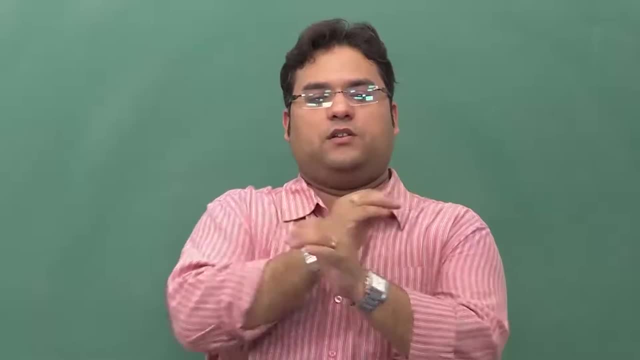 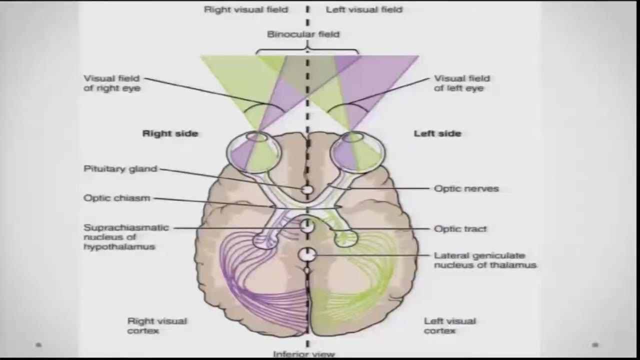 which is basically the retinal part. ok, So the inward part, basically, is where this crossover is happening, and so input from one eye is going to another hemisphere, input from the say, for example, input from the left eye, is going to the right hemisphere, input from the right eye is going to the left hemisphere. 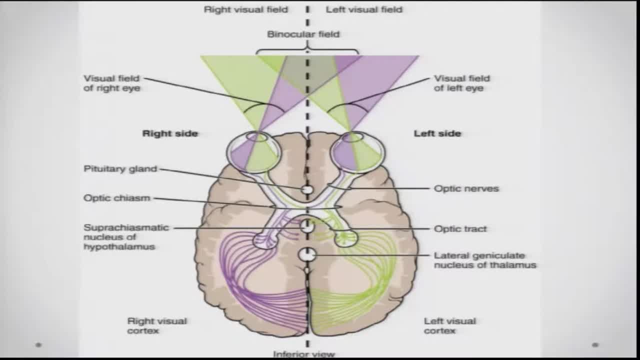 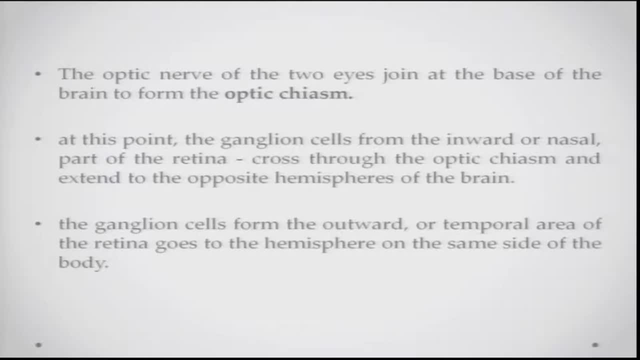 this crossover point is called the optic chiasm, Just going back. so at this point, at the optic chiasm, the ganglion cells from the inward or the nasal part of the retina cross over. through the Optic chiasm, extend to the opposite hemisphere of the brain. the ganglion cells from the outward 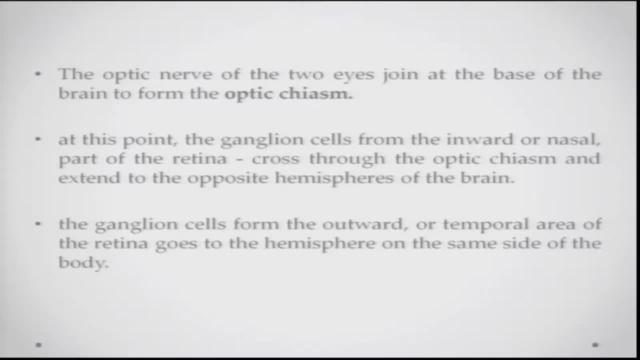 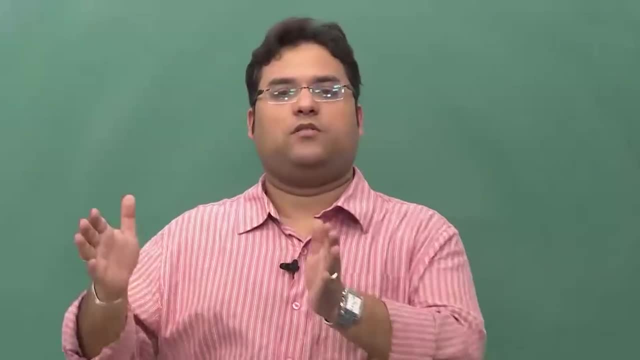 or the temporal area. So the inward area is called the nasal area, the outward area is called the temporal area, which is actually near the temples. the temporal area of the retina goes to the hemisphere on the same side of the brain. So this is how this crossover happens. 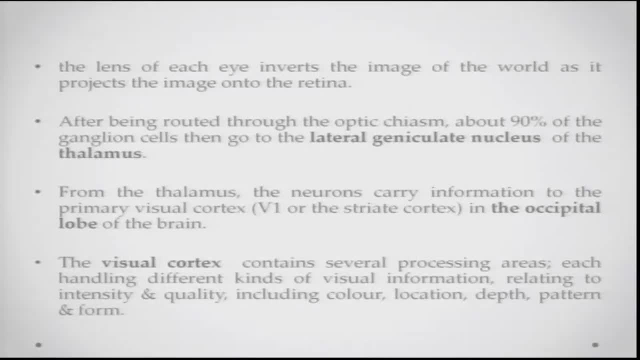 The lengths of each eye basically inverse the image. So you might have done elementary physics in your class 6th or 7th. you might have known that a particular lengths kind of forms. It is an inverted image of the world as it projects this image. and the same happens with 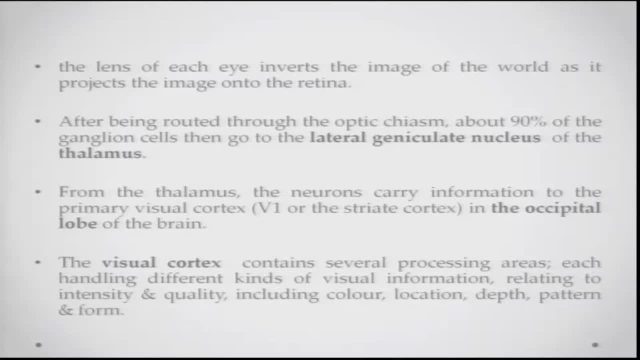 the lengths of the eye, So it projects an inverted image to the retina. after being routed ah through the optic chiasm, about 90 percent of the ganglion cells then go to what is called the LGN, or the lateral geniculate nucleus. ah, this is a set of nuclei in the thalamus. ok, 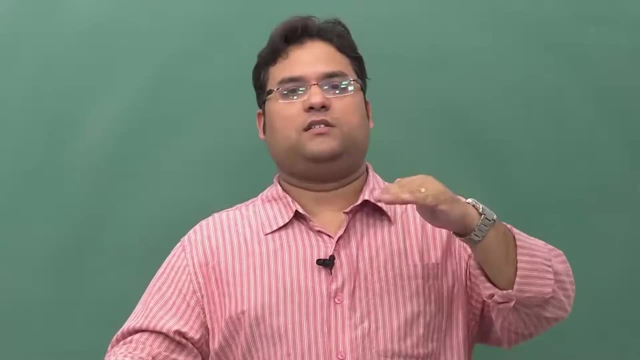 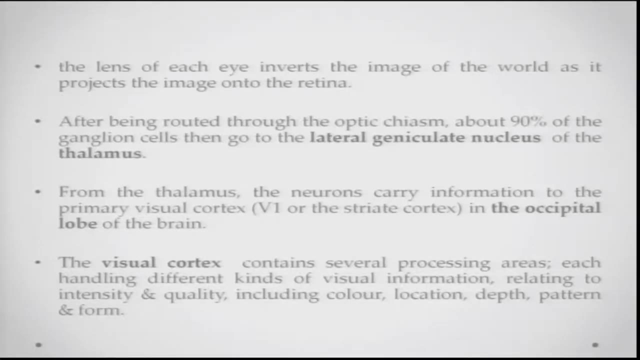 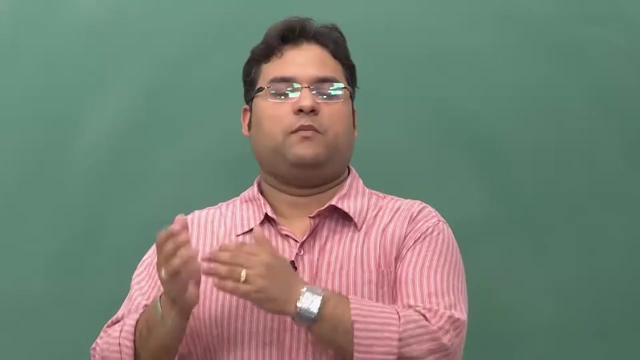 So thalamus is the basic region of the brain wherein this is going to. from the thalamus what happens is The neurons carry information to the primary visual cortex, which is the first area in the occipital cortex that kind of receives this information, the primary visual cortex in the 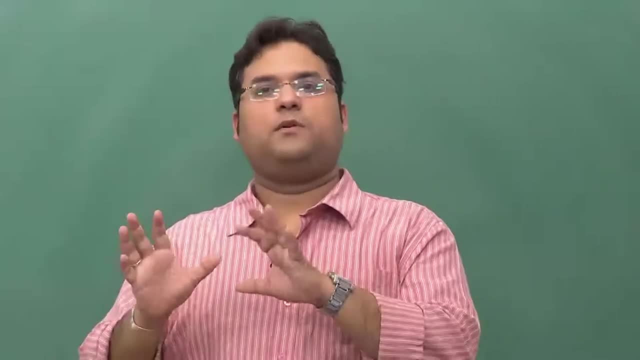 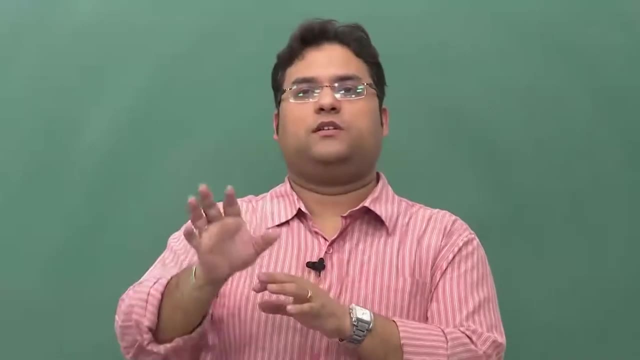 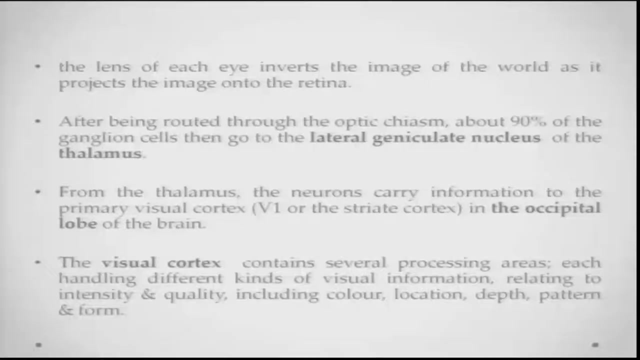 occipital lobe of the brain. and this occipital cortex, basically, is where the detailed processing of this information coming from these, you know, from the retina, starts to happen. ok, So this visual cortex or your occipital lobe, ah, 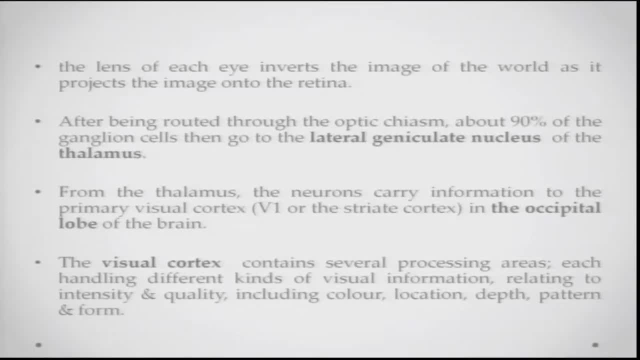 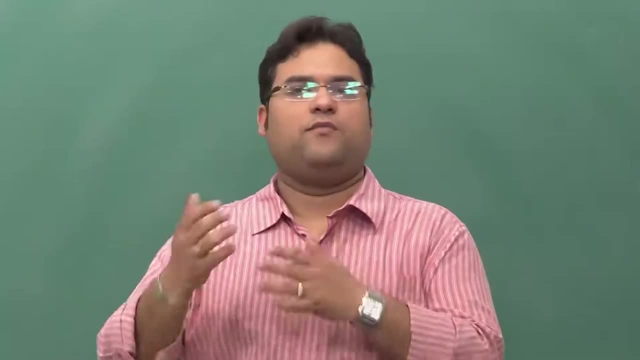 So these several ah processing areas, each of these areas ah really carry out, ah you know, different kinds of analysis on the incoming visual information, ok, And these areas can differ into how they process the intensity of light, how they process the quality, how they process the color, the depth information, the location of something, the 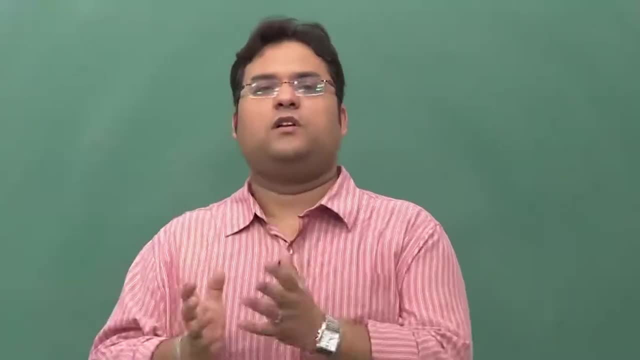 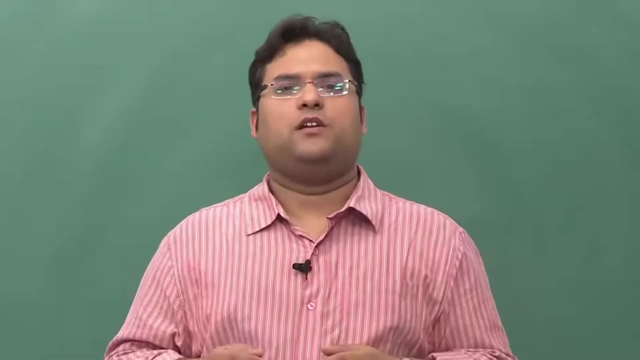 kind of pattern there is ah. the form there is: see visual ah. perception is a really complex activity. I can take an example. I can say that if I am looking towards you, I am actually looking at ah, multiple levels of information. I am looking at colors and 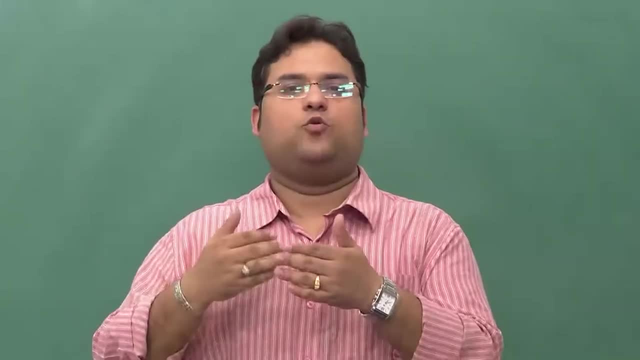 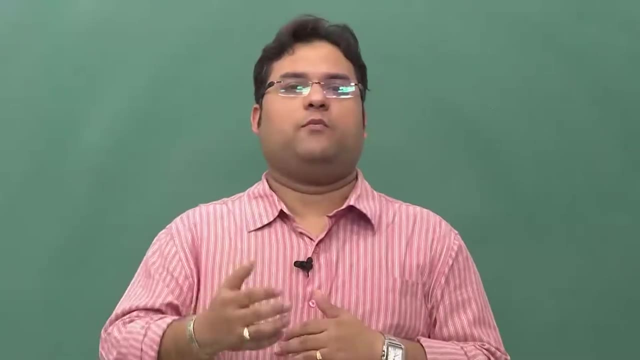 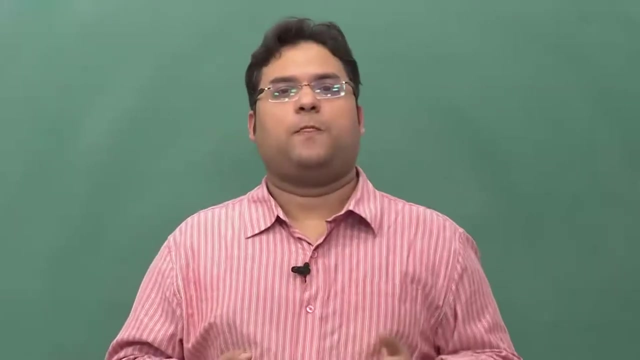 looking at contours, that are shapes. I am looking at whether it is a two dimensional or a three dimensional image, So I am looking at depth as well. I am making sense of how far you are, ah, from me. ah, that is distance, ah, So I am doing, ah, and I am also say, for example, processing whether you are moving or not, isn't? 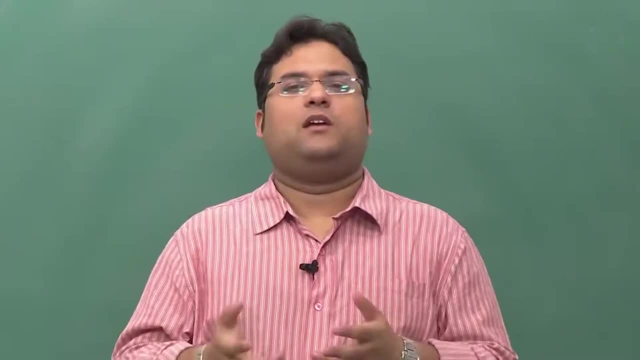 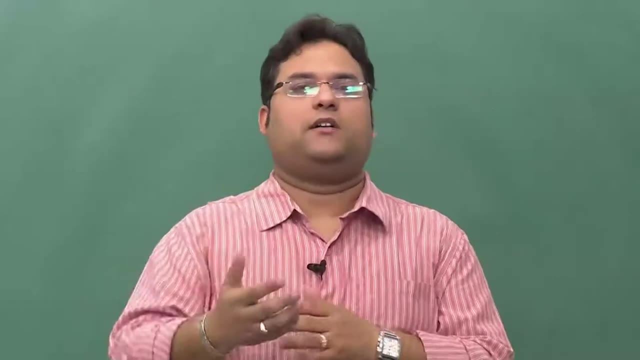 it. So, even though visual perception- ah, you know, typically might seem rather simple, but there are So many processes happening at the same time with anything you are looking at. So if you look out and you are kind of able to figure out that you know there is car moving. 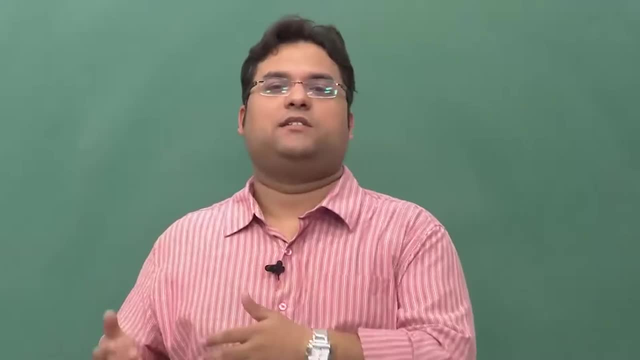 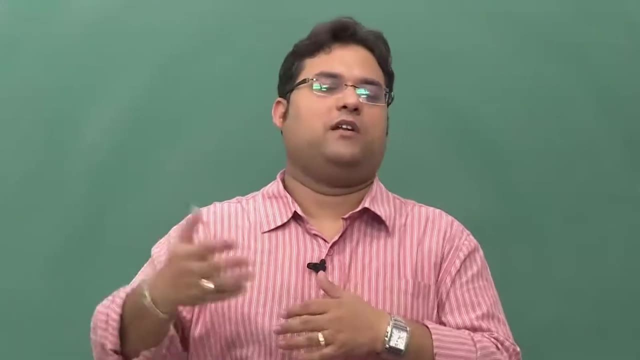 on the road. ah, you are actually doing lot of these analysis over there. you, you know, you have the basic shape of the car, you have the colors, you have, ah, the information that is just moving you have you might get to know that. you know, ah, what kind of car it is. 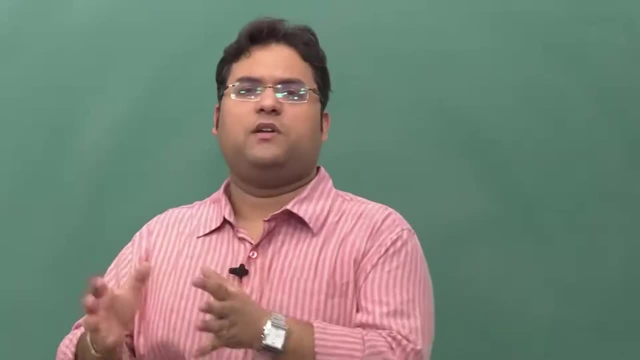 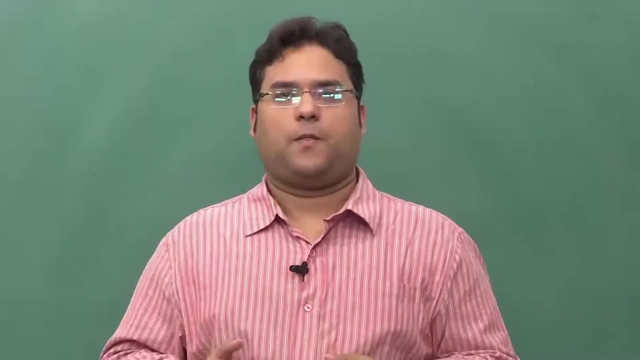 So you kind of doing that kind of analysis as well. So you are doing these multiple levels of analysis on whatever visual information is ah coming ah to your eyes, ah via light. Let us have a look at this figure. This is how, ah you know, this is ah really, you know, arranged. 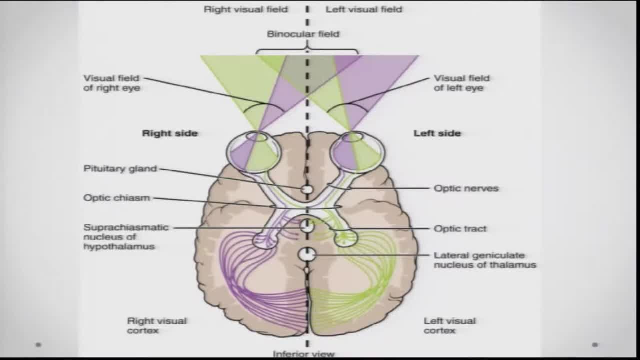 So, ah, you have a binocular field where in both eyes are getting the input, but you also have, ah, the right visual field and the left visual field. ok, So, right, visual field is predominantly ah, basically, what the right eye is looking at, left vision field isициate down the other left eye is looking at. you can see here in: 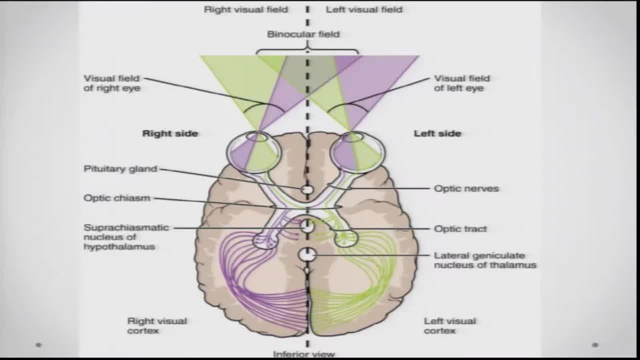 this figure that So Radielek dot glo EPA. information from each of the visual field goes directly to the contralateral hemisphere. Contralateral is basically the other side of the optic chiasm. So you can see in this figure the information in the right visual field goes first to the 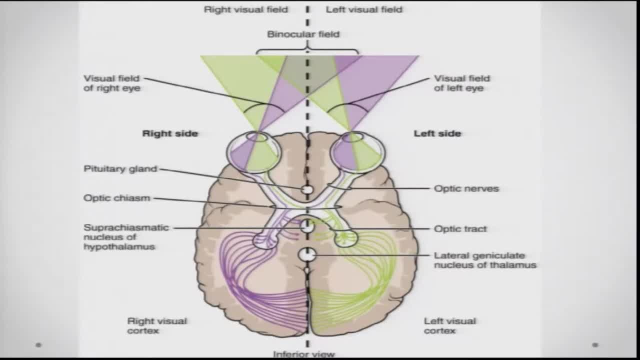 left visual cortex, the information in the left visual field goes first to the right visual cortex. I am saying first because generally these contralateral connections of these ganglion cells are supposed to be are found to be faster than the ipsilateral. basically the same side. 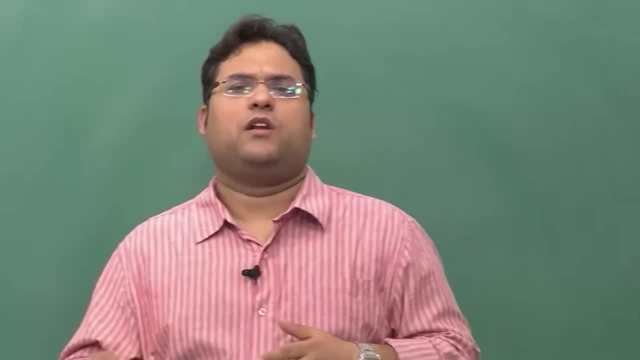 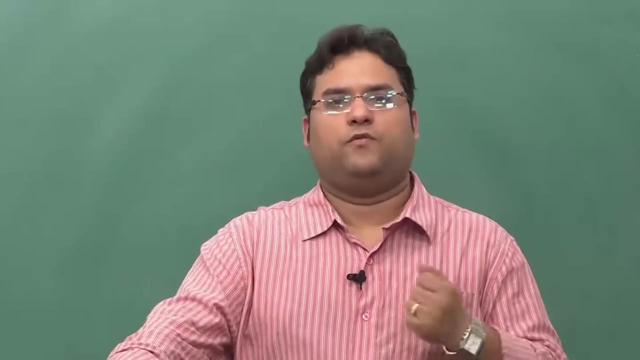 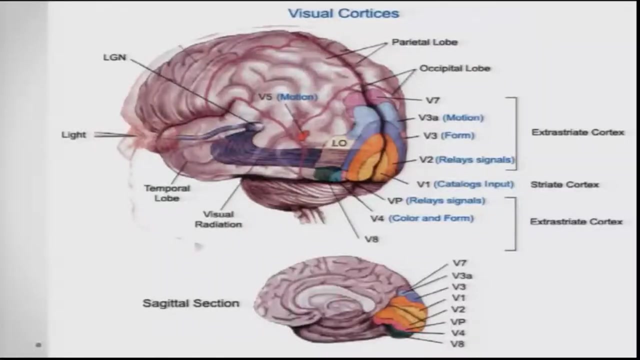 connections. So this kind of also leads to really interesting or important effects. we will talk about them in due course, when we are actually talking about more things about visual perception. For reference, here is the figure which presents what is called the visual cortices. 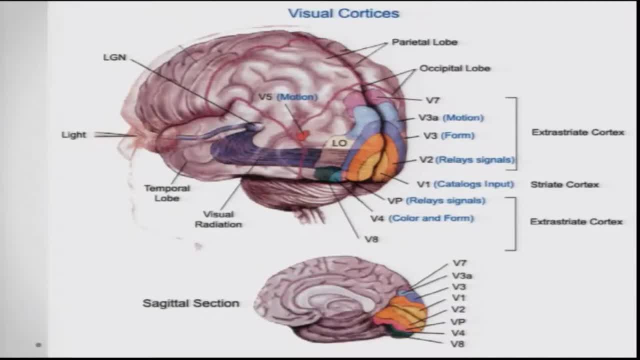 You can see that there is this lateral geniculate nucleus which is connected to the brain. You can see, light is entering through the eyes. it is kind of, you know, through the optic nerve reaching This area called the lateral geniculate nucleus. that is what your thalamus is about and from 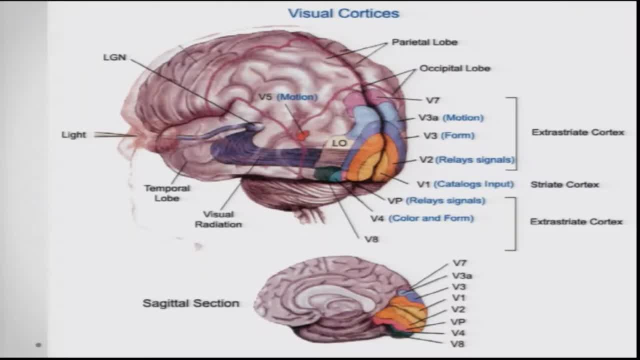 there the information is being relayed to what is called the occipital lobe, which is the lobe which has to do with vision, and you can see these so many areas here. Each of these areas are referred to as so V1 to V8. you can see, and you can see what. 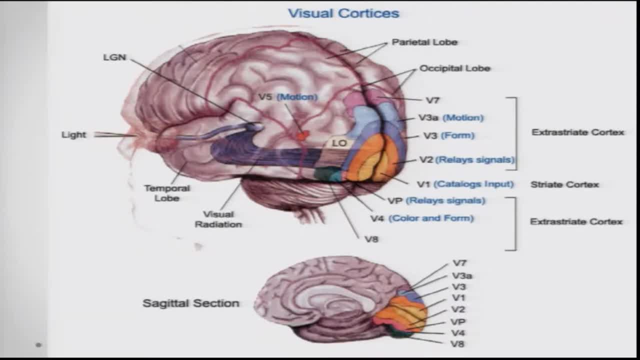 these what the specializations of each of these areas are. See for example, I am just reading out for you: Areas from: V1 basically is called the visual cortex. Basically it is called the striate cortex. It catalogs whatever input is coming in. area V2, basically is you know more responsible.